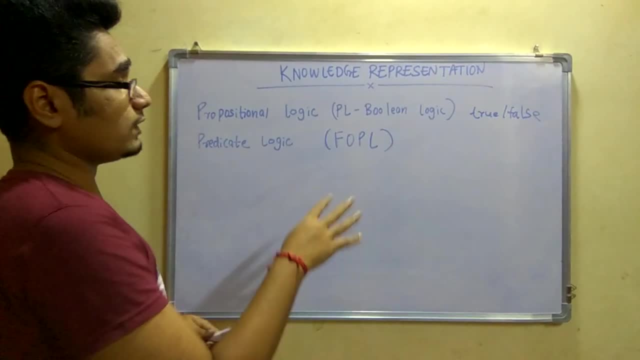 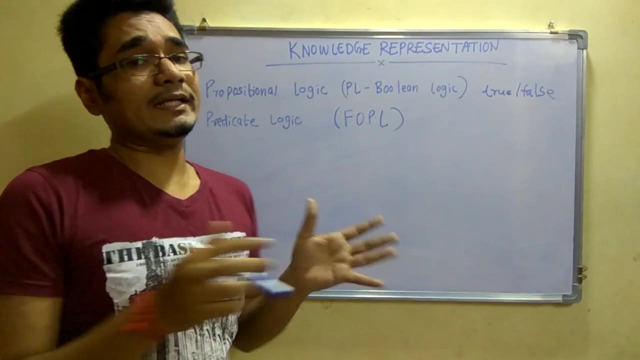 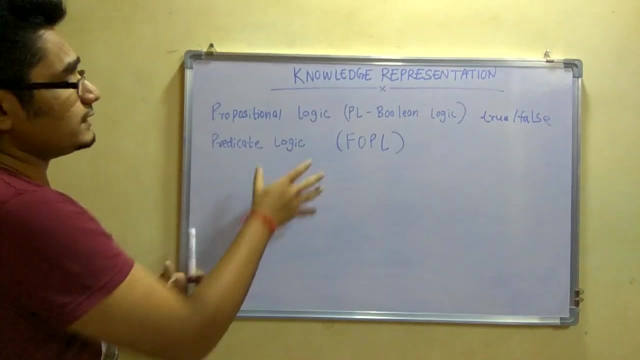 Next is the predicate logic, also called as the first order predicate logic. It has got three main types: First argument, second argument, as well as the third arguments. So we will be covering that in our example section. So to get a brief idea about predicate logic is that: 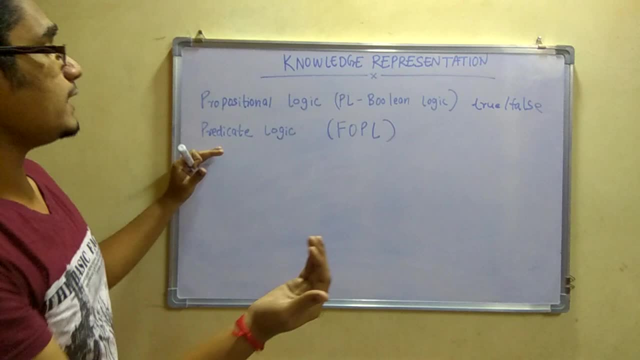 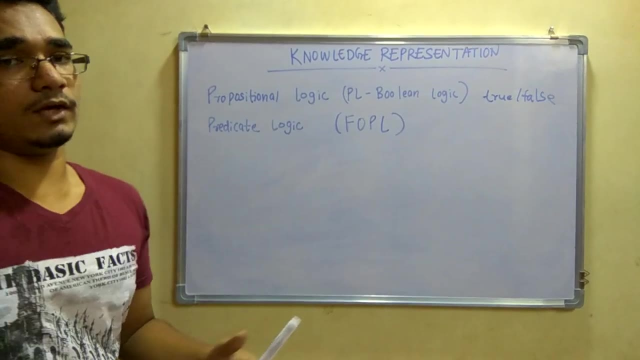 predicate logic is a superset, or it can be considered as a superset. It is a superset of propositional logic. So what? all things which comes under propositional logic is segregated into predicate logic. So let's get started. So here is an example. 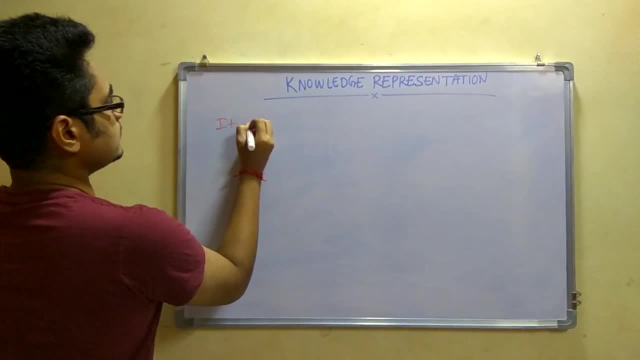 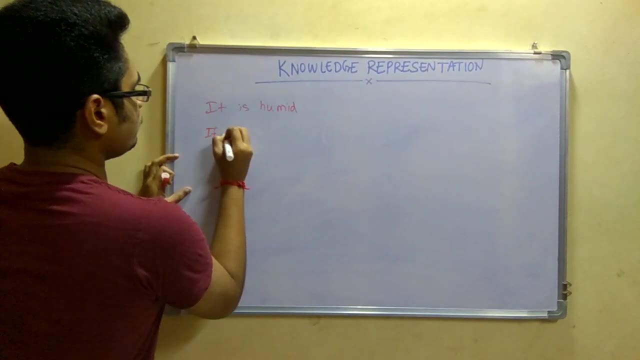 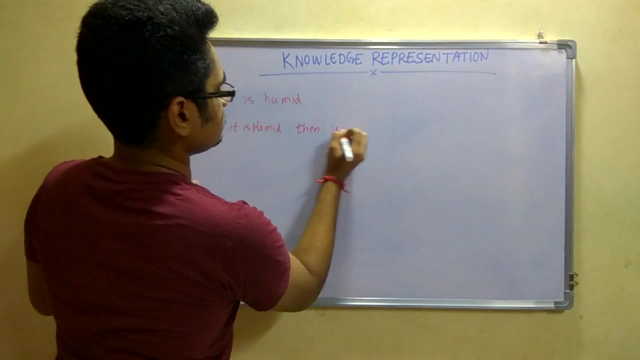 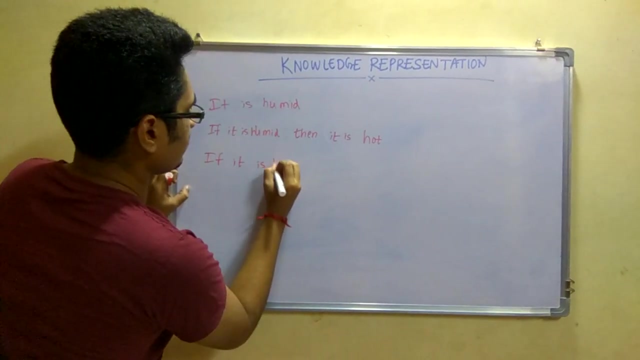 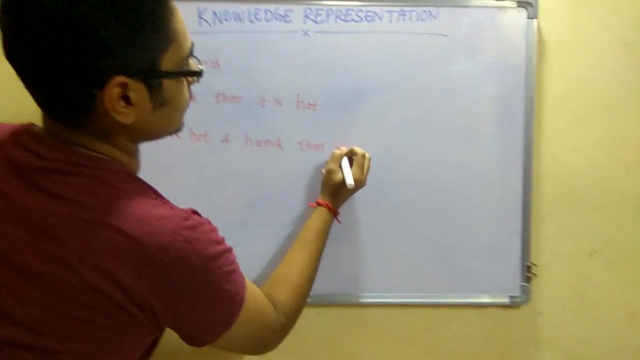 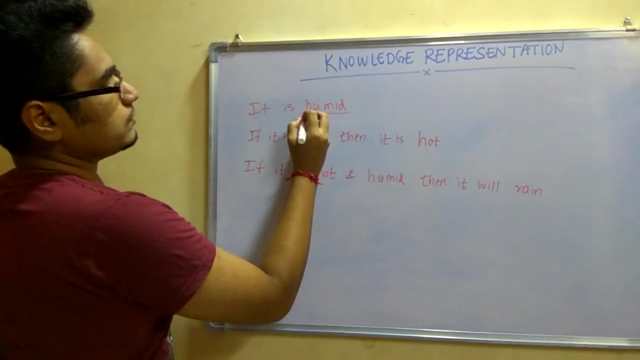 Suppose I want to represent. it is humid, For example. it is given three statements: It is humid, and if it is humid then it is hot. And one more is there: If it is hot and humid, then it will rain. Now for humid. now you have to see the object. if it is humid, 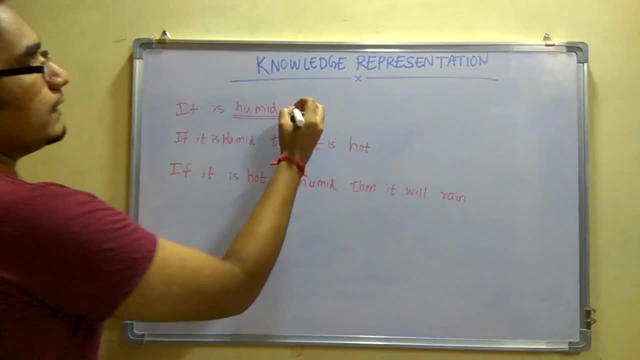 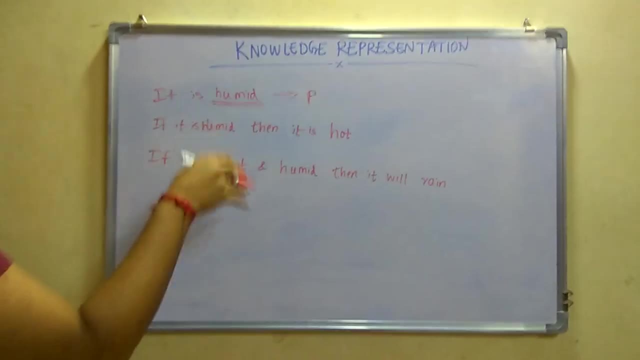 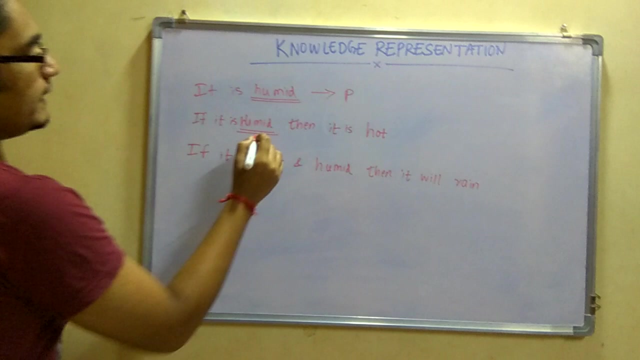 Now for this statement. for basically humid, we will assign Q. Sorry. P means P represent it is humid. Now let us go to the second statement. If it is humid, then it is hot. Now, this statement says that if it is humid, that is, if it is P, then it is hot. 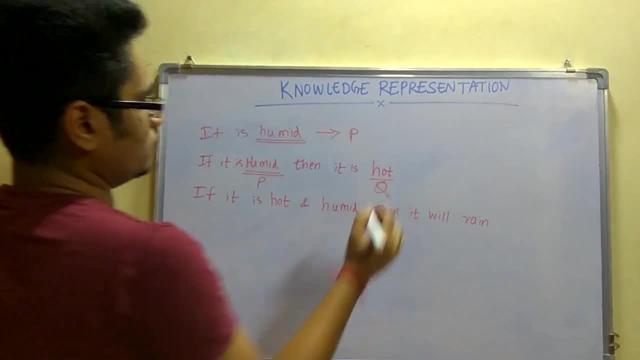 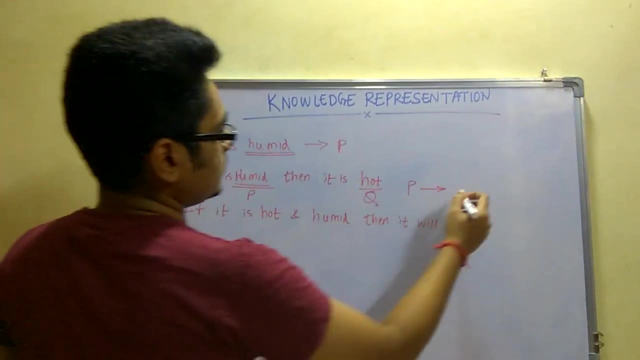 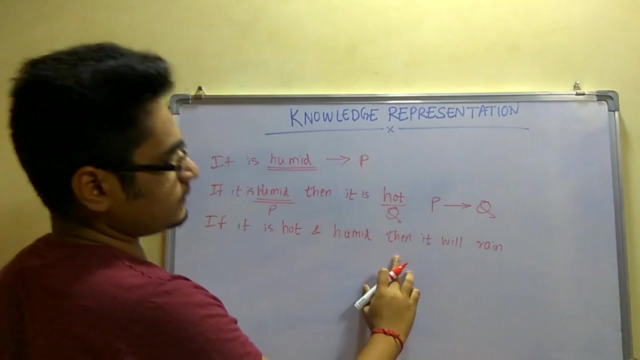 So for hot, we will represent Q. So this statement basically tells that if it is humid, that is, if it is P arrow, then it is hot. Now this arrow represents then. So if it is humid, then it is hot. Next, if it is hot as well as humid, then it will rain. 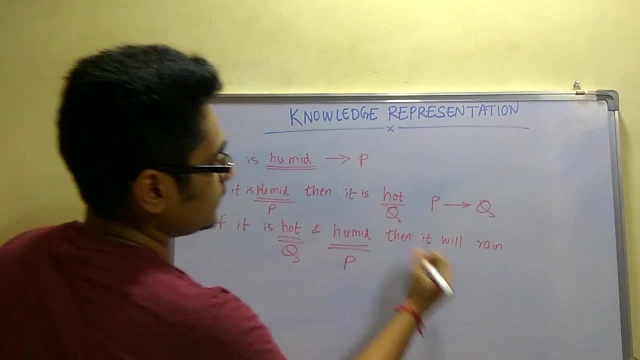 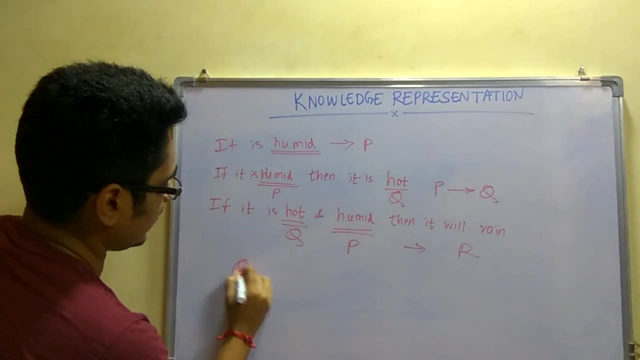 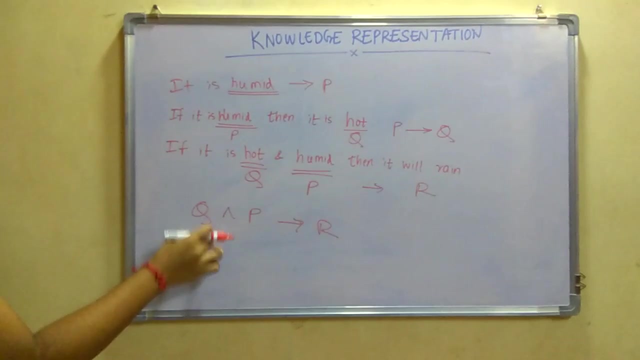 First is hot, that is Q, and humid, that is P, then it will rain. That is, for rain will give R. So basically it goes like this: Q as well as P gives R. Now the statement tells that it should be hot as well as humid for it to rain. 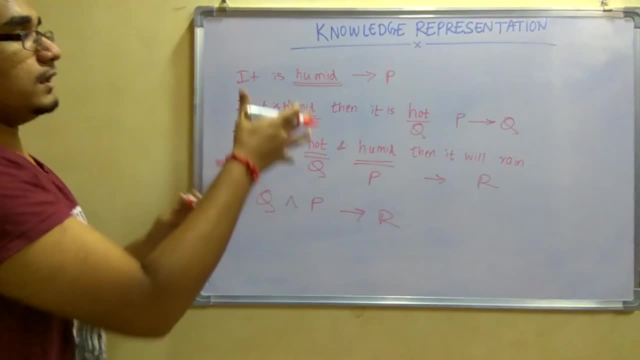 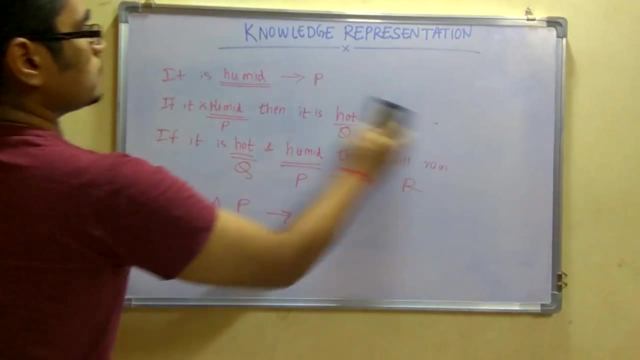 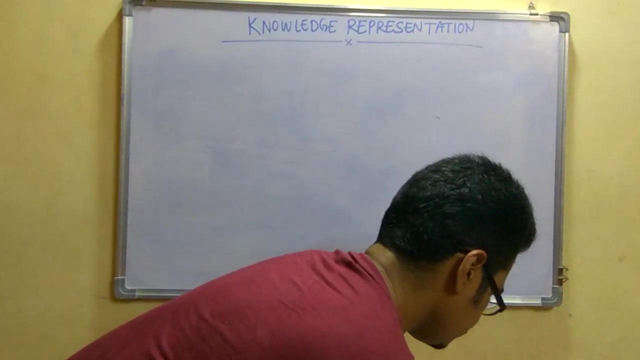 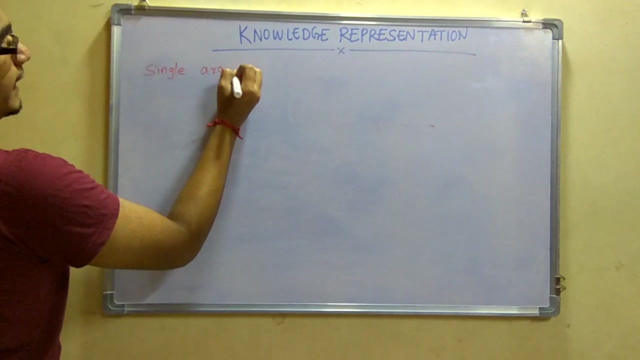 So Q and P gives rise to R. So this is what is the propositional logic. So next is the predicate logic. So, to go with predicate logic, there are three main types of predicate logic Now. first is a single argument. predicate means only one argument would be there. 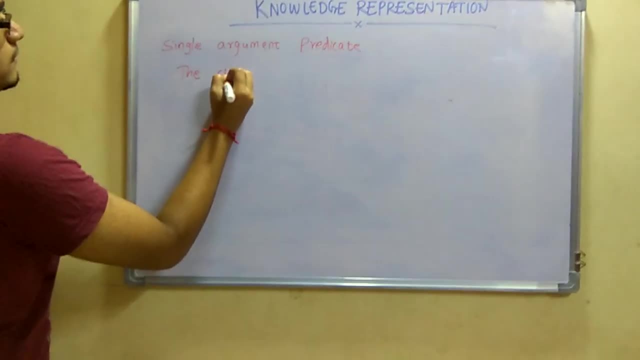 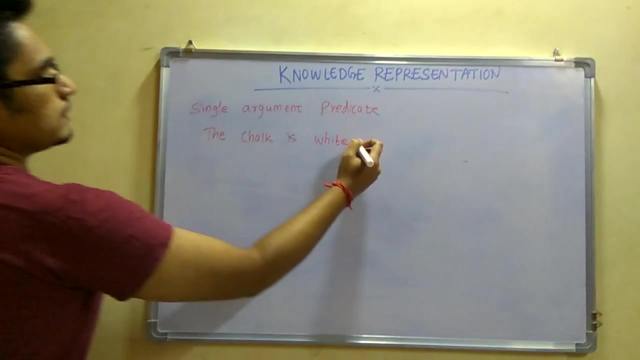 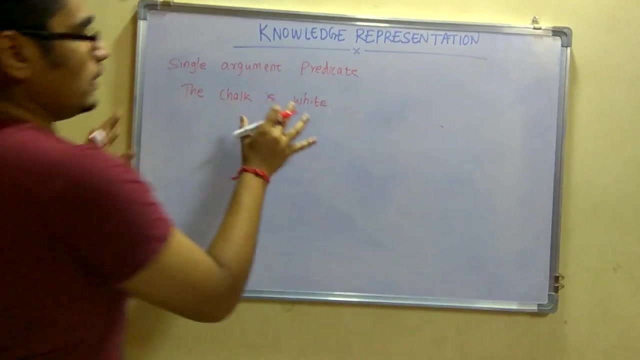 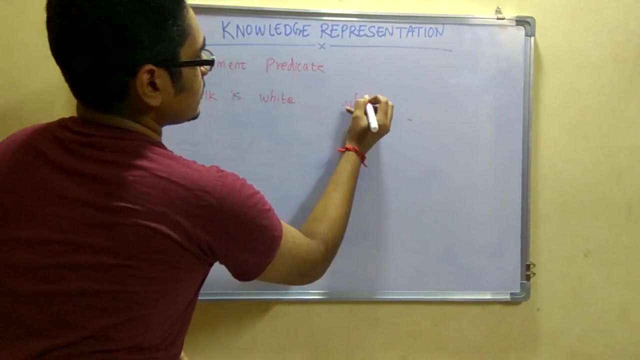 Means that, for example, consider: the chalk is white. Now in this, if you go by the basic English means, you can understand that the chalk is a noun and white is an adjective. So while representing in predicate logic, or when you will be converting into logic, you will be writing like: white means the thing is white. 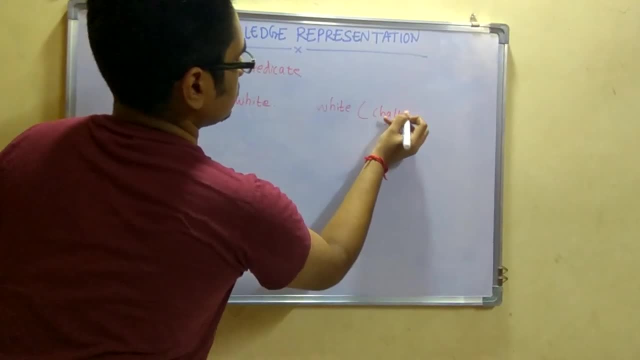 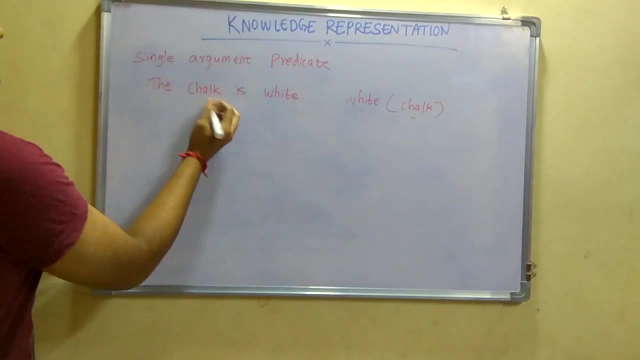 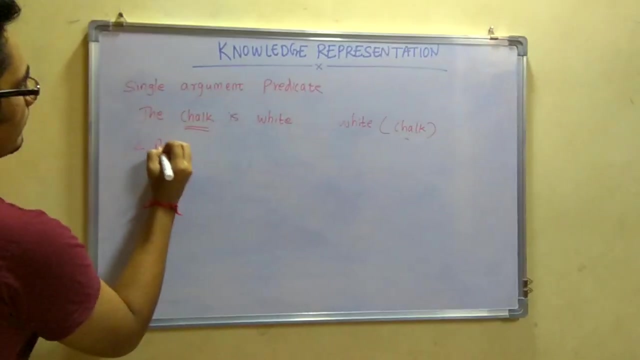 The object is white, So the object would be chalk. Means the chalk is white, So this gives rise to single argument. Means only one argument is there, that is chalk. So chalk is our argument. Next is the two argument predicate. 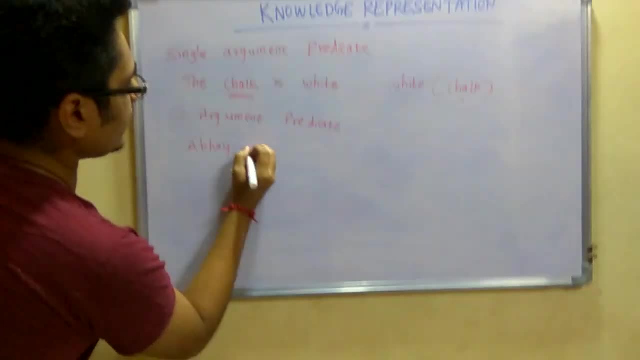 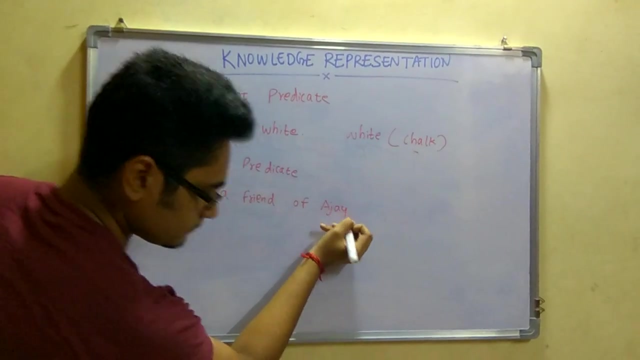 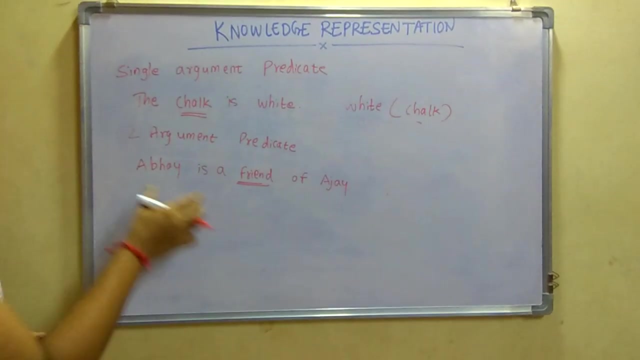 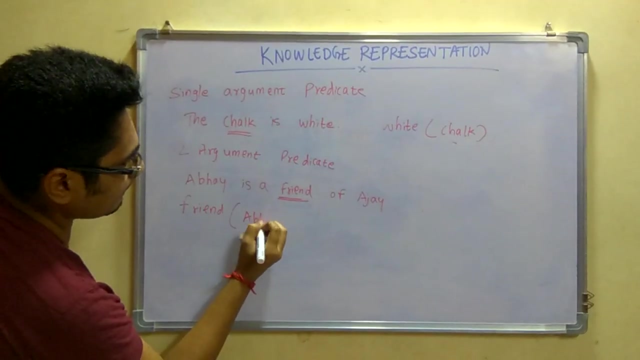 Now in this the statement would be: Abhay is a friend of Ajay. Now in this, friend would be the describing thing or this, basically the connecting link between Abhay and Ajay. So we will be writing friend in bracket, Abhay, comma, Ajay. 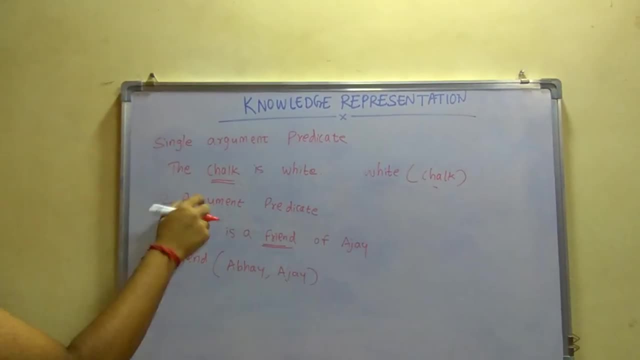 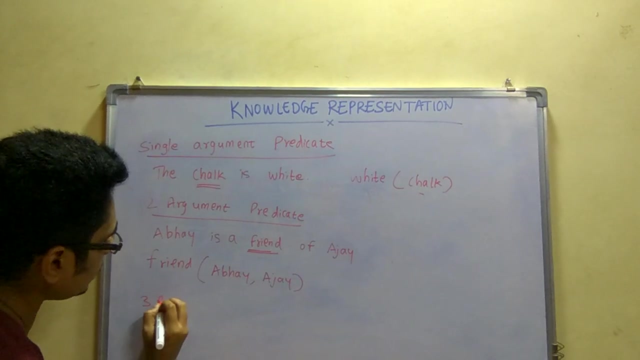 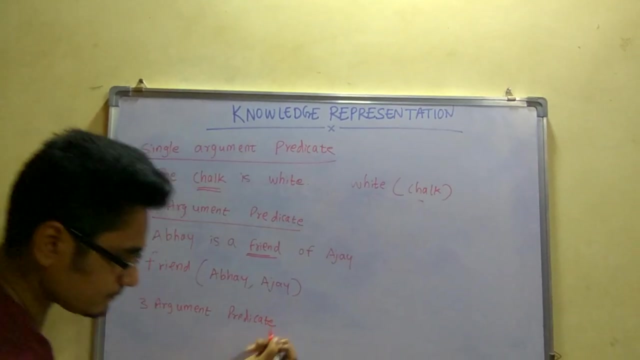 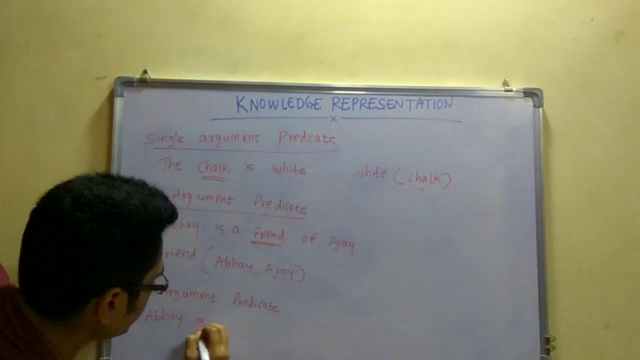 Means. in this two arguments are there, So that's why it is a two argument predicate. and in this, one argument is there, So it is a single argument. Next, we have three argument predicates. Now. in this it will be like Abhay gave a book to Ajay. 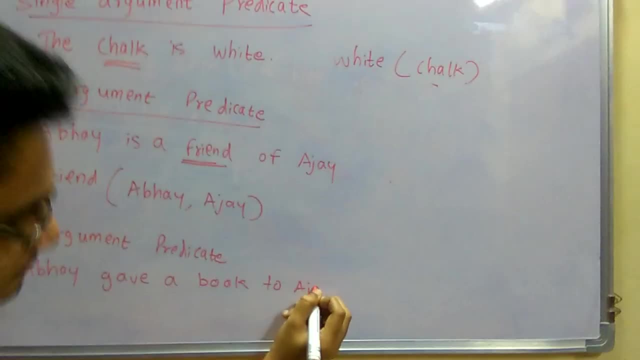 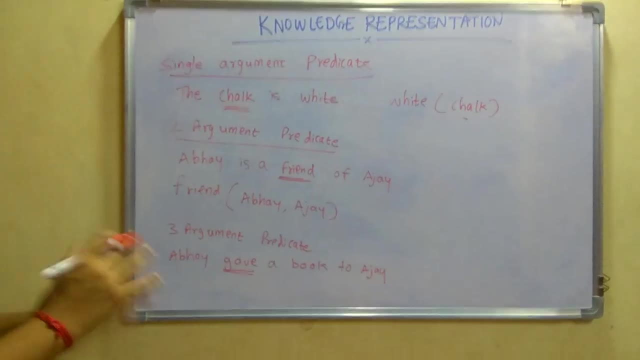 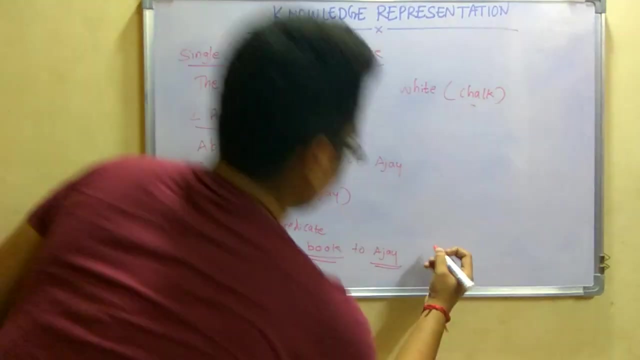 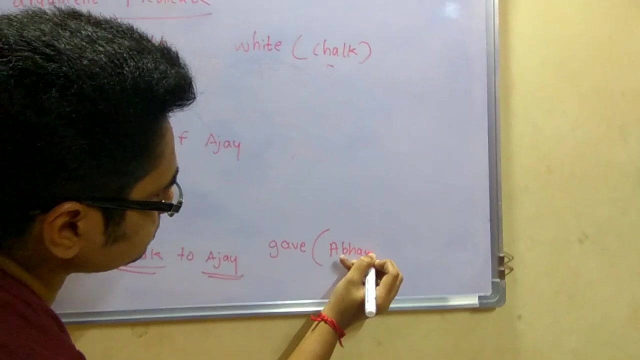 So in this give will be the connecting link, Means Abhay gave a book to Ajay. Abhay is a noun, Book is also a noun, Ajay is also a noun. So we will be writing like give, and first it will be Abhay, then comma, book and Ajay.